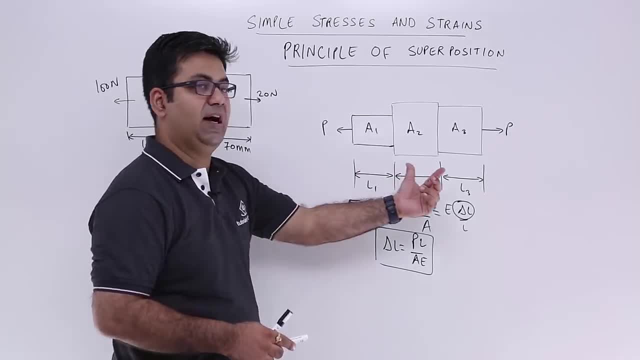 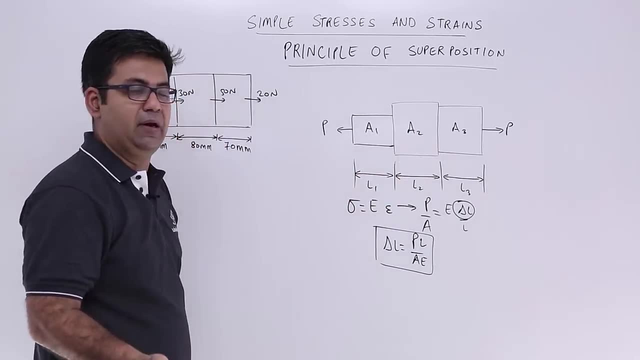 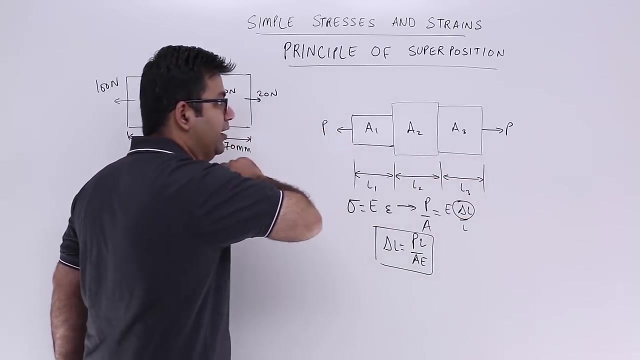 Now, in this kind of a problem, you have a stepped shaft or it can be a stepped bar. You have different areas. If you have a stepped shaft, you will have different diameters. Different diameters will produce different areas, But the entire material or the entire body is acted upon by the same amount of loading on both sides. 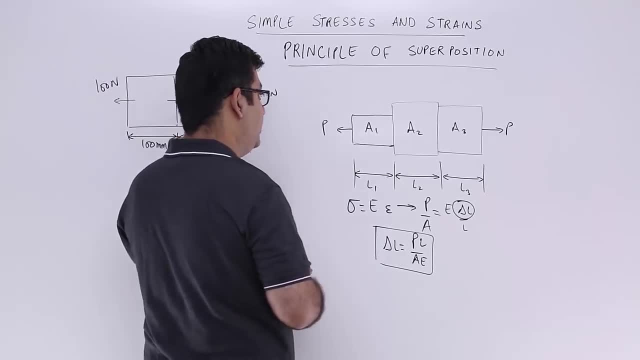 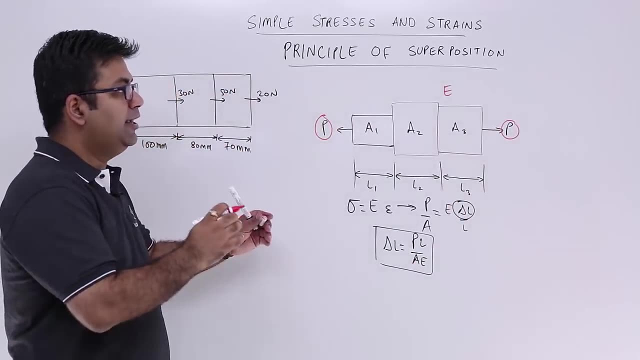 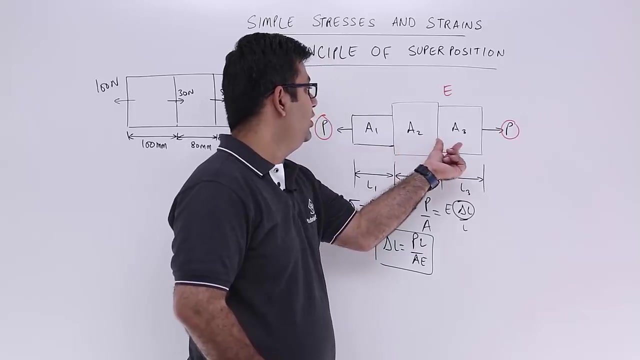 The material is also the same. So in this case the load is the same, The load is same and the material is same. So p and e will be same. This means p is acting on area a1.. It is acting on area a2 and it is also acting on area a3.. 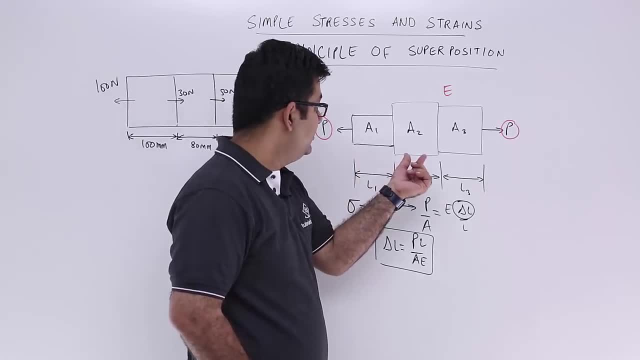 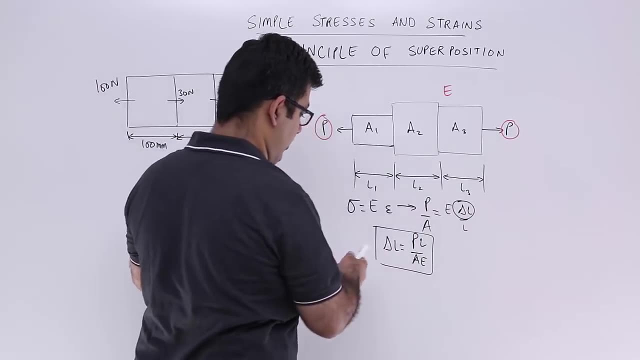 So elongation in this section plus the elongation in this section plus the elongation in this section would be the total elongation for the entire body. So the elongation in section, I would say this is section 1.. This is section 2.. 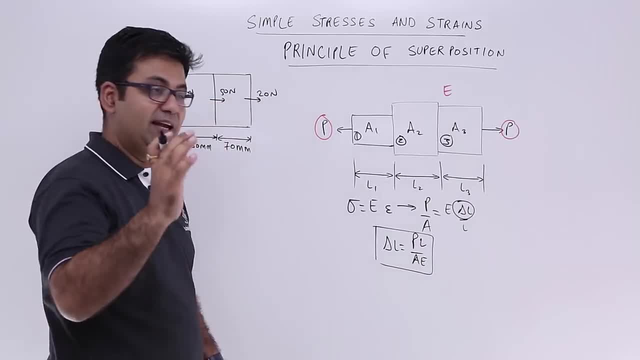 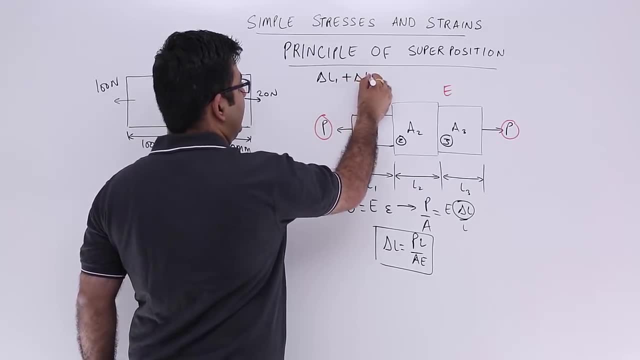 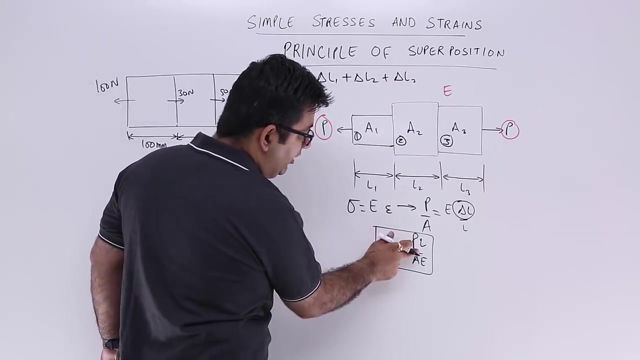 And this is section 3.. Elongation in section 1 is delta l1. Elongation in 2 is delta l2. And elongation in 3 is delta l3.. So what is delta l1?? It will be p l1 upon a1 into e. 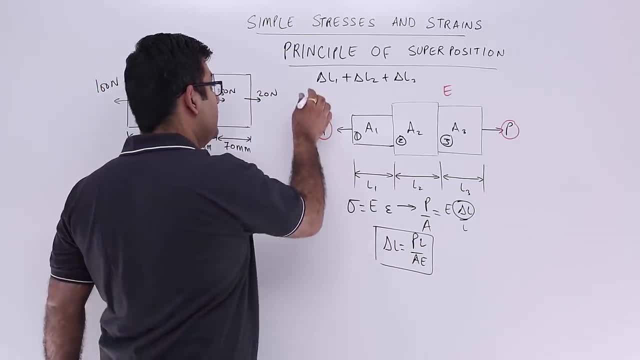 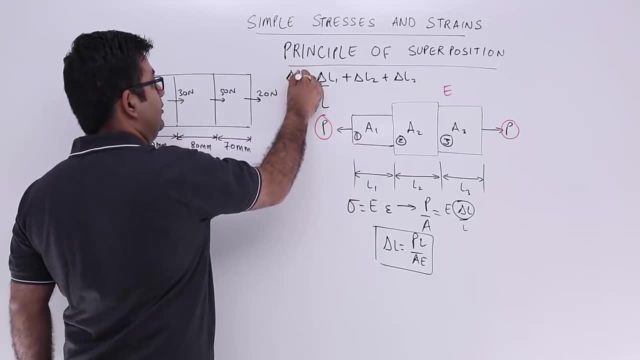 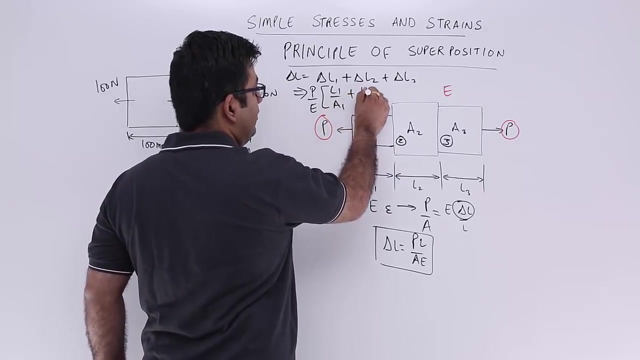 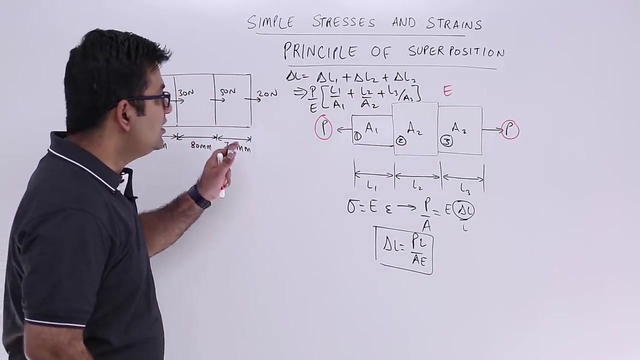 Now p and e are same, So I can take out p and e to be constant or common values. This is equal to delta l, So this becomes l1 upon a1 plus l2 upon a2 plus l3 upon a3.. So this is how you apply the principle of superposition in such a scenario. 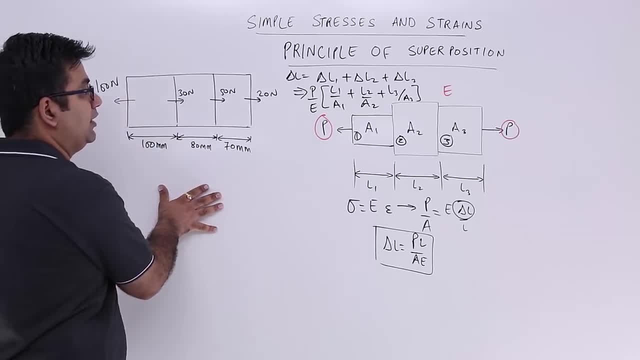 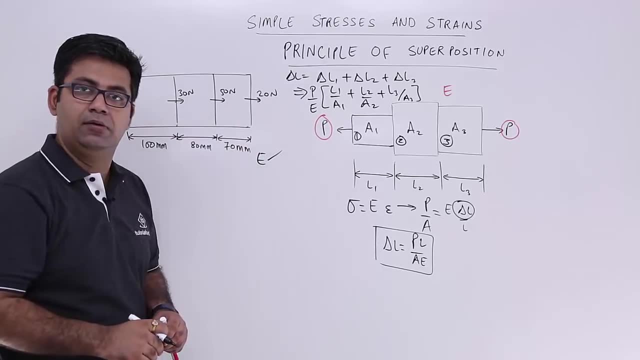 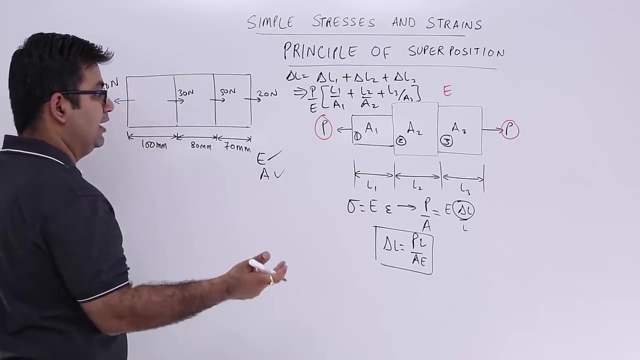 Now a more challenging scenario occurs when you have a problem like this. In such a case, yes, the Young's modulus is same because it is a same material. The diameter would be the same or the cross section area would be the same. That becomes easy. but in this the load is not same. 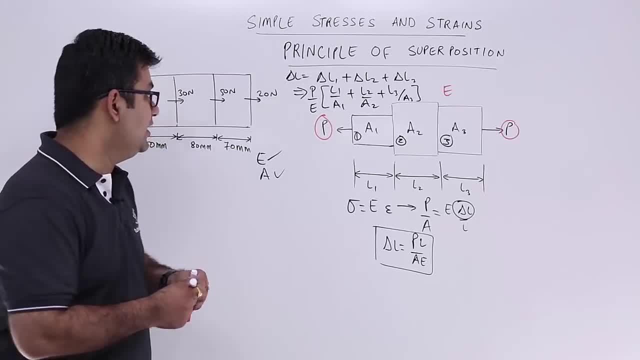 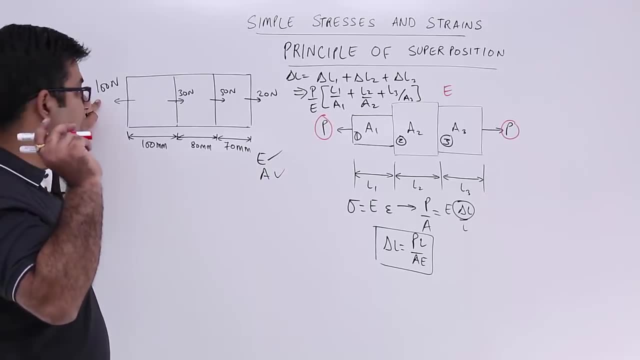 And length is, but obviously not same as well In this case. first of all, look at the equilibrium of the entire body. You have a load of 100 N towards the left hand side. You have a load of 30 on this section towards the right. 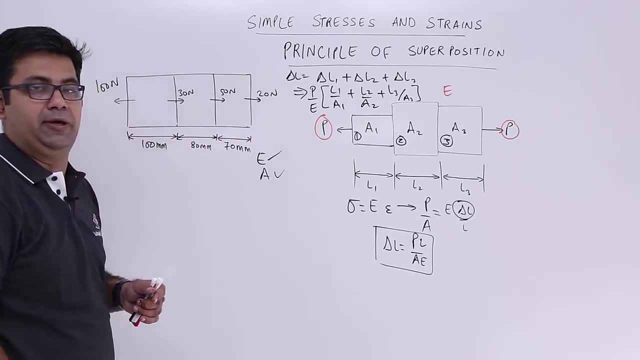 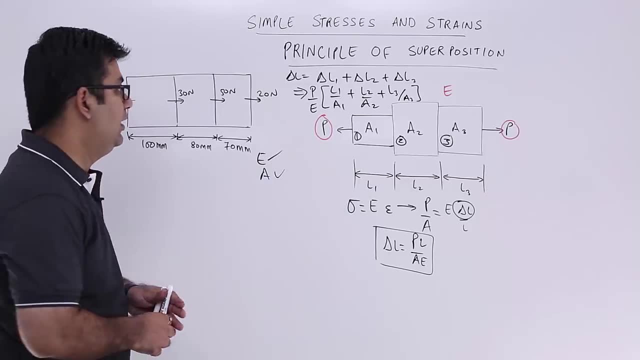 50 on this section towards the right and 20 on that towards the right. The equilibrium means the net left hand side force is equal to the net right hand side force. You will have: 100 is equal to 30 plus 50, which is 80 plus 20, which is equal to 100.. 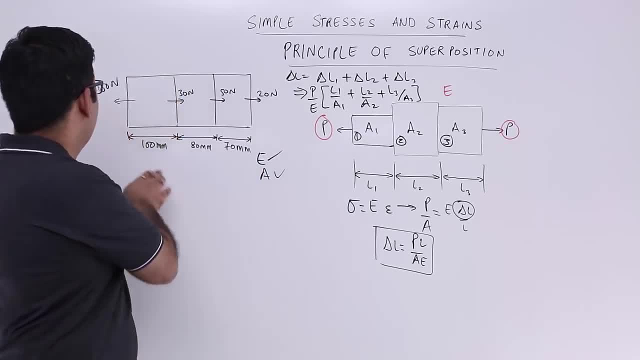 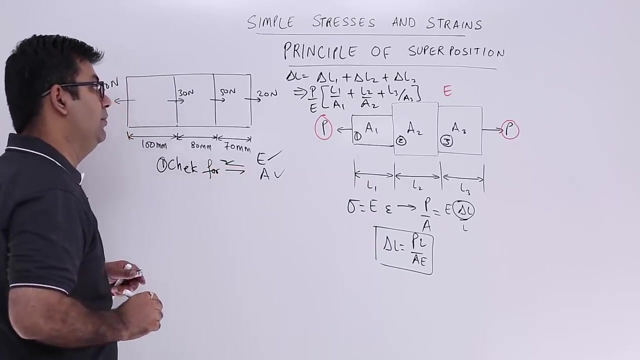 So in this case the total force towards the left side is equal to the total force on the right side. So that is a very good thing to have. So first of all, check for equilibrium. So this is an equilibrium: 100 is equal to 30 plus 50 plus 20.. 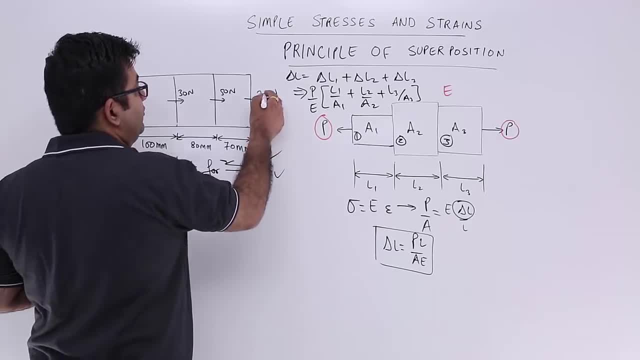 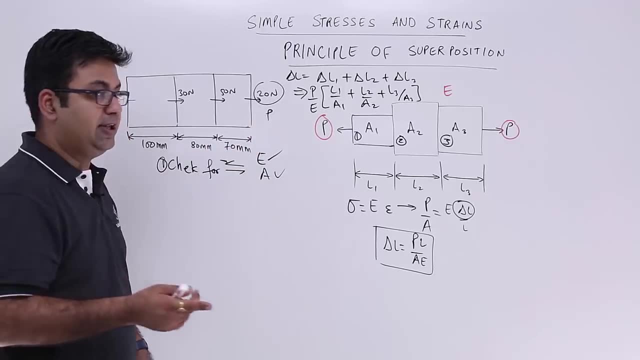 Another variation that you can have. You might not be given this force. You might be only given P over here. So this becomes an unknown force Before you find out the net elongation or the net change in the length of this beam or this bar. 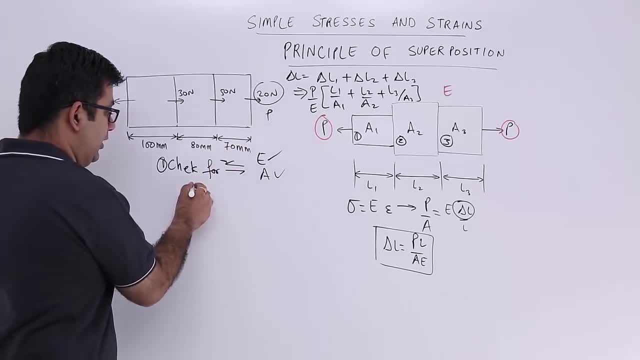 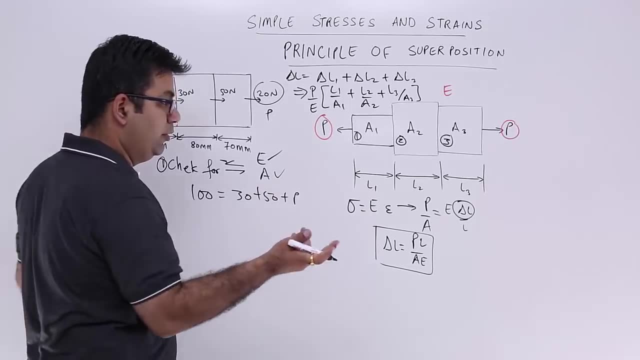 You have to find out P over here. To find out P, you will say: 100 is equal to 30 plus 50. Plus P, So P from here would be 20.. So this is another variation that you can see in this kind of a question. 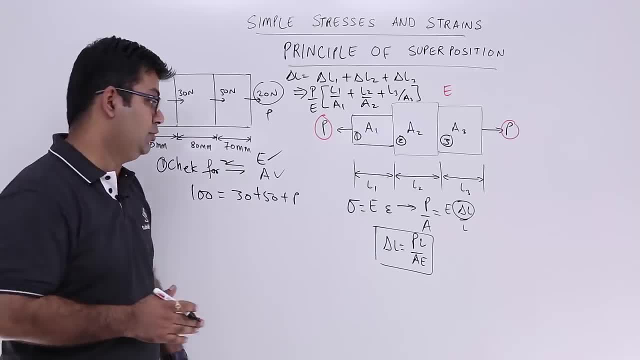 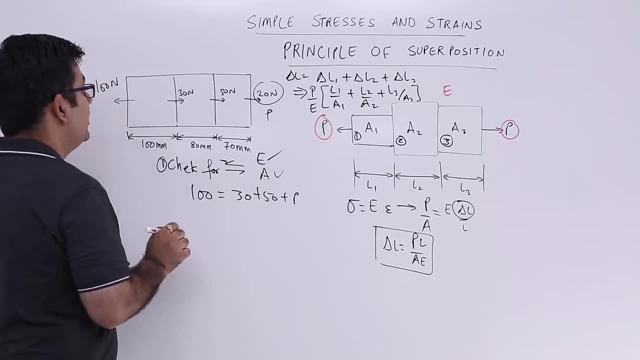 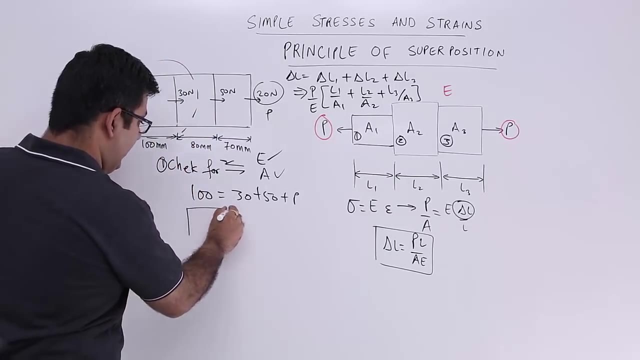 Now, the very first thing in such a question: you should check this. The second thing would be to create sections in equilibrium. Let's first of all take this section. So this is a section of length 100 mm. Always consider the lower force. 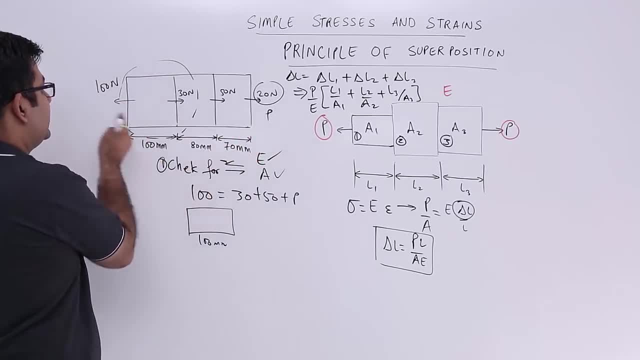 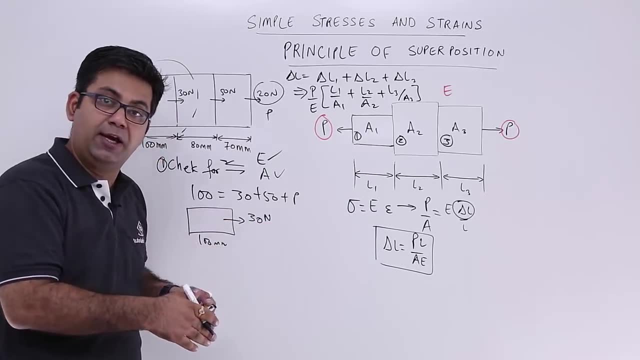 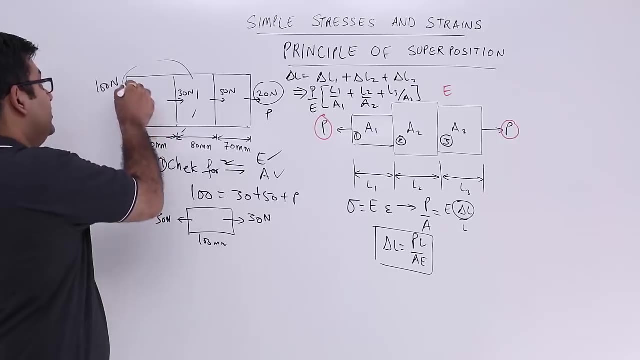 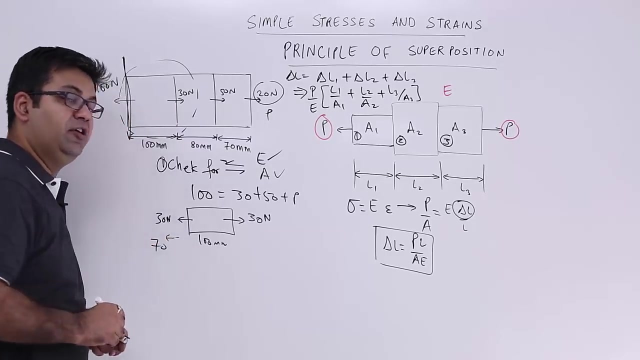 So in this section you have this as 30 and this as 100.. I will always take the lower force and apply 30 N over here To bring this section into equilibrium. I will have to apply 30 over here as well. On this particular section, that is, this left hand section, I still have a surplus of 70 N. 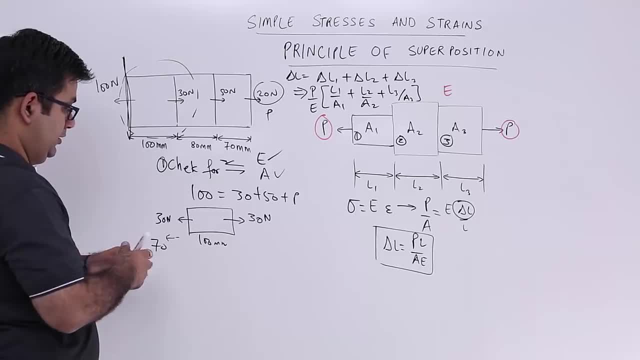 Now, what will I do? I will take this section, This entire section, This and 50.. So what will I do? I will draw a figure below this. Now, the length is 100 plus 80. So this becomes 180 mm. 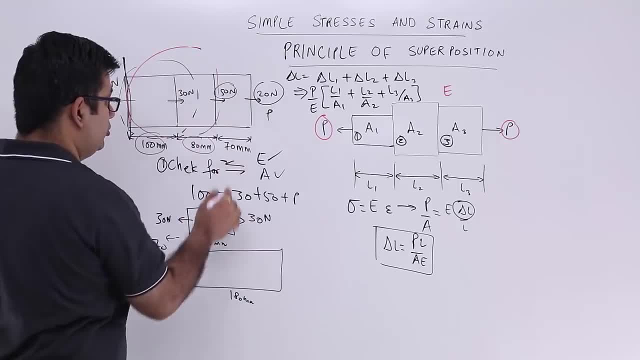 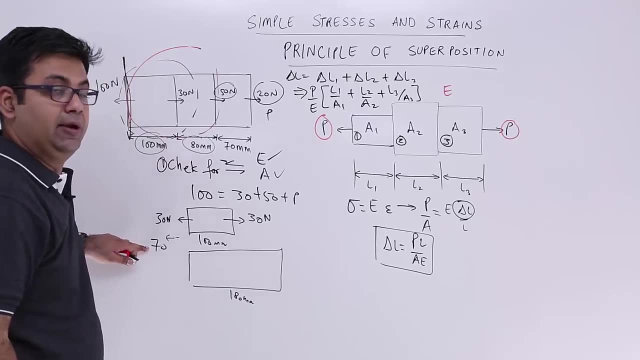 Again taking the lower force, because from 100 I have already consumed 30 over here, So now I only have 70 over here. So still 70 is higher as compared to 50. So I will apply the lower force, which is 50 over here. 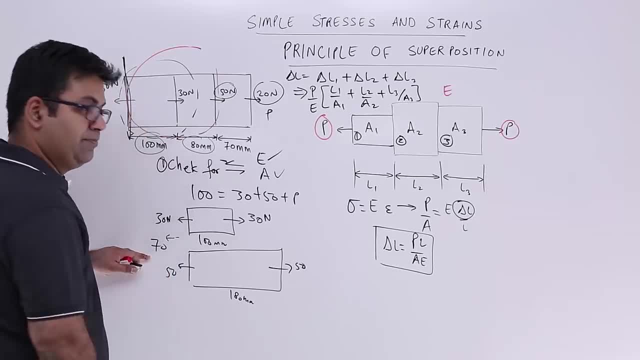 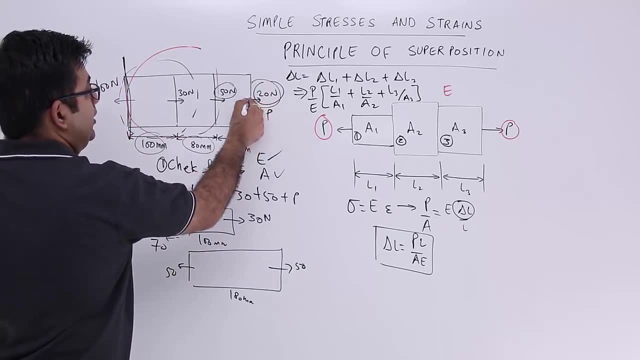 Out of 70, I will apply 50 over here. So now this section comes into equilibrium. Now, still, I have 20 surplus. Is that right? And that 20 can be put into equilibrium with the last section. So I will increase the section length. 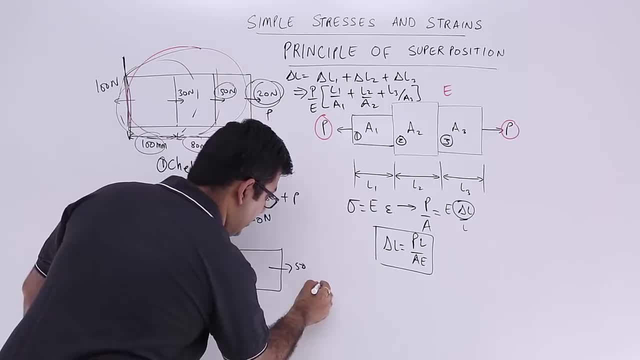 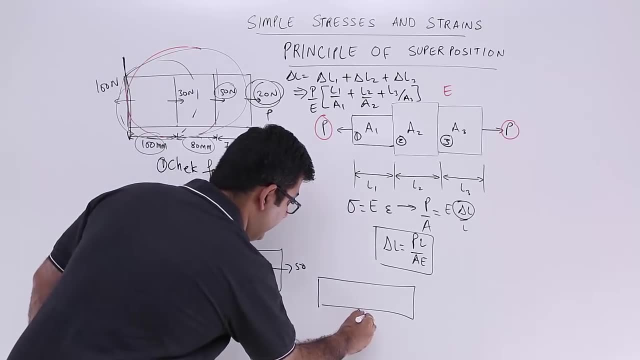 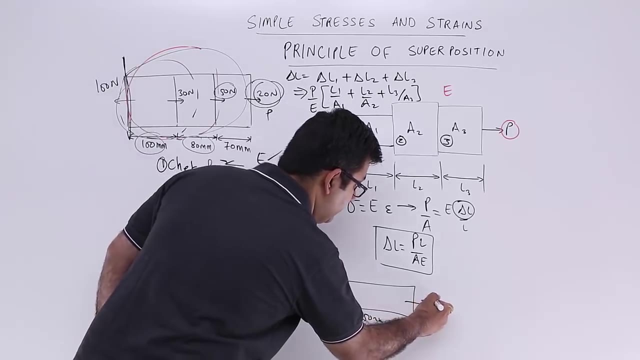 I will take the entire case. So this would be equal to this complete value. So this length is 100 plus 80 plus 70, which is 250.. So this is 250 mm. This is 20, which came from this deficit or this surplus, and this is also 20.. 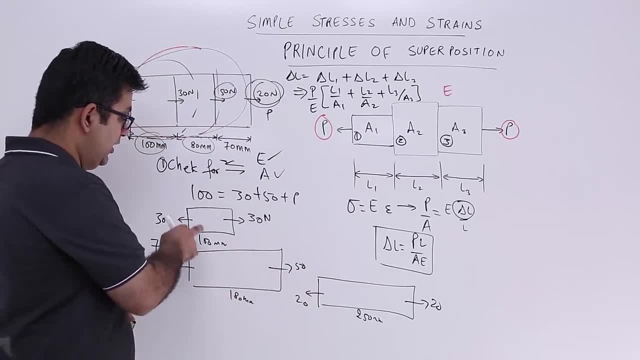 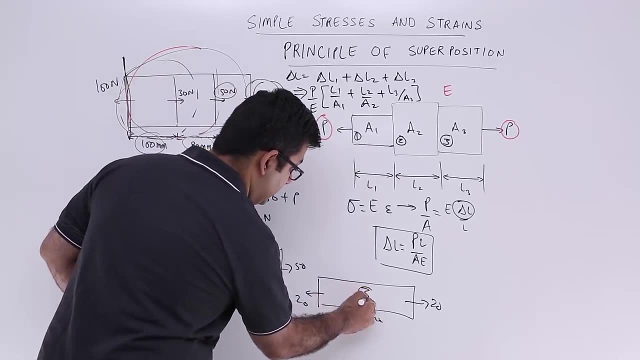 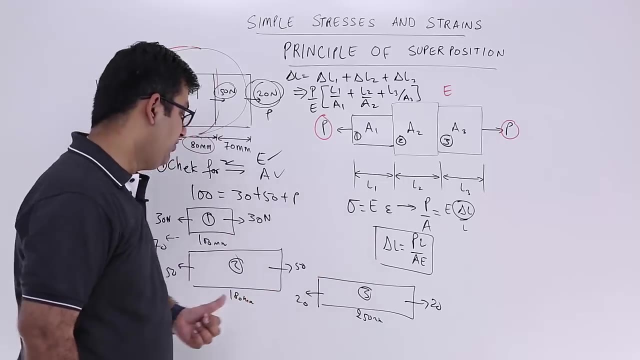 So now you have 3 sections. In both these sections, equilibrium condition is existing, So this is section 1.. This is section 2 and this is section 3.. Alright, The area is already same. I will apply this equation to find out the net elongation. 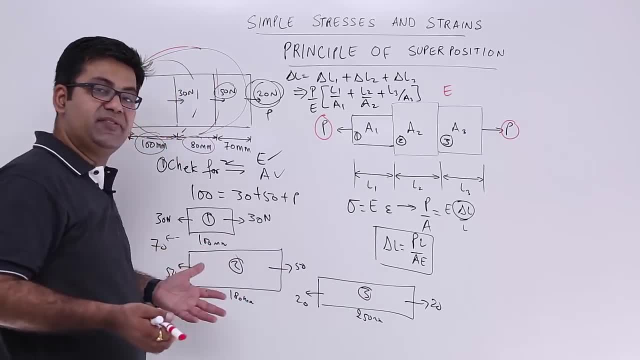 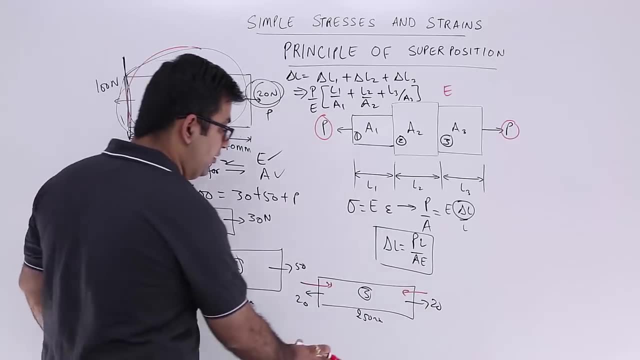 The net elongation or the total elongation. There might be a case where you will have one load acting in the compressive direction. In that case you will have a contraction in this case and the elongation in the rest of the two cases. 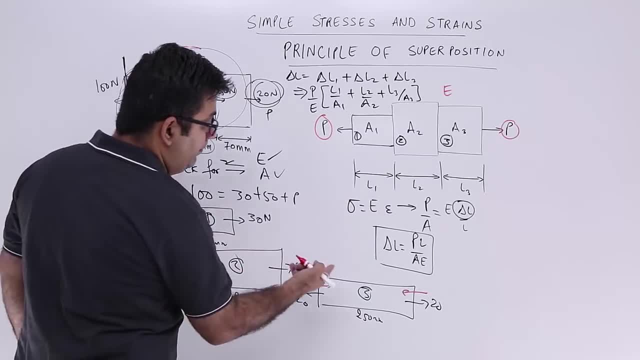 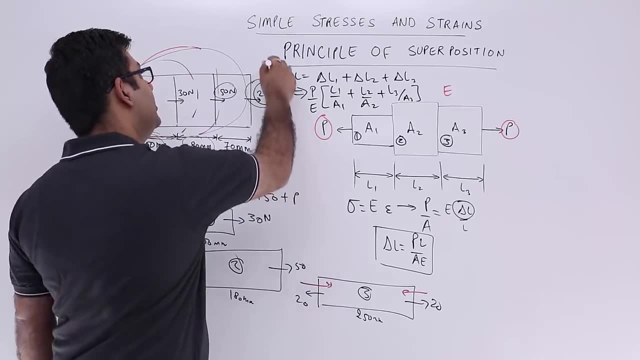 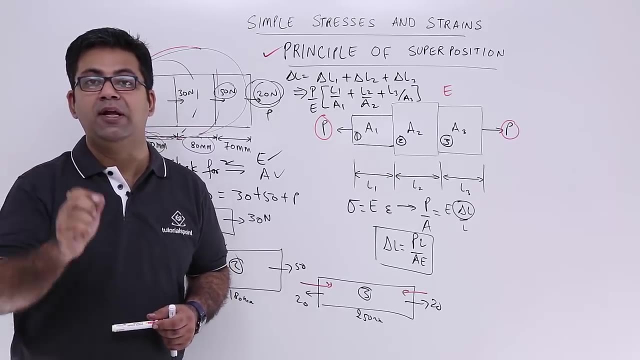 So you will have delta L1 plus delta L2 minus delta L3.. Okay, So this is how you solve these kind of questions, by the application of principle of superposition. Now let's move on to the next topic and talk about thermal stresses. 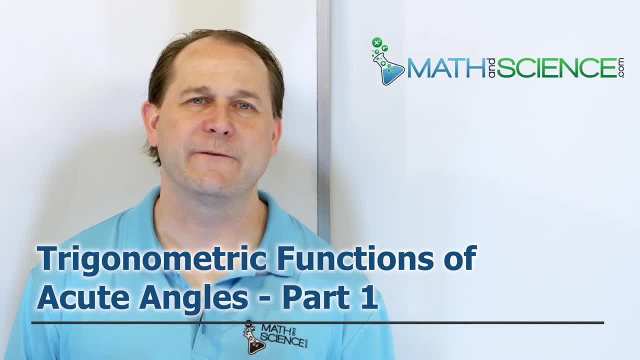 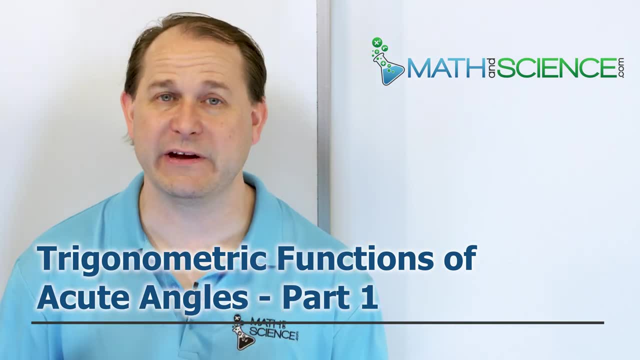 Hello, welcome back. The title of this lesson is called Trigonometric Functions of Acute Angles. This is part one- Really complicated sounding title, but I promise I'll break it down for you so it will be very easy to understand. So we have to introduce all of the trigonometric functions.